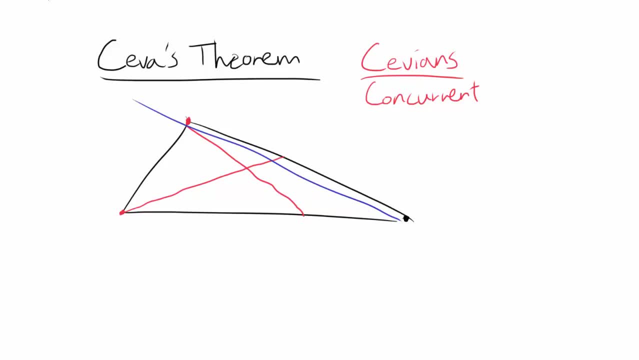 If you draw it like this, they are not going to intersect at the same point. But when you draw this sievian through the intersection of the original intersection of the first two sievians, you have all of the sievians intersecting at the same point And you call this concurrent. Concurrent means three or more lines. 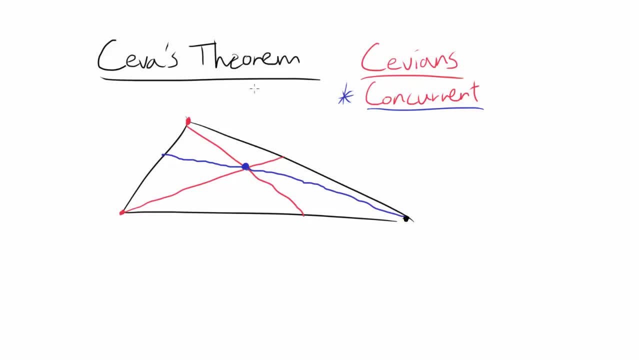 are intersecting at the common point. So Sebas theorem tells you the necessary and sufficient condition for this thing to occur. So let me label this a bit- A, B, C. And what you're going to do to show that all three sievians are going to be concurrent is like this: Let's go around You. 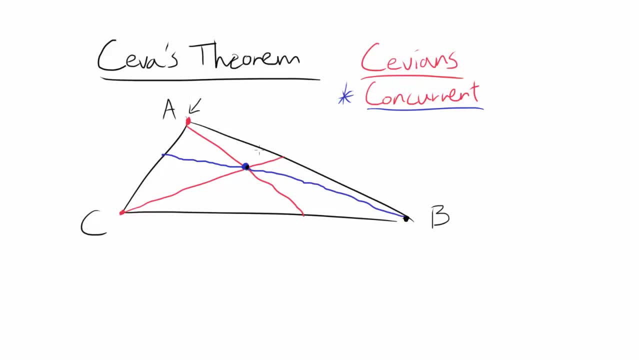 pick a point to start with. I pick vertex A, just for the sake of it, And you're going to pick a direction to go, And I pick this direction And you're going to go around the triangle. You're going to go around the triangle And you're going to come up with some ratios that you're going to. 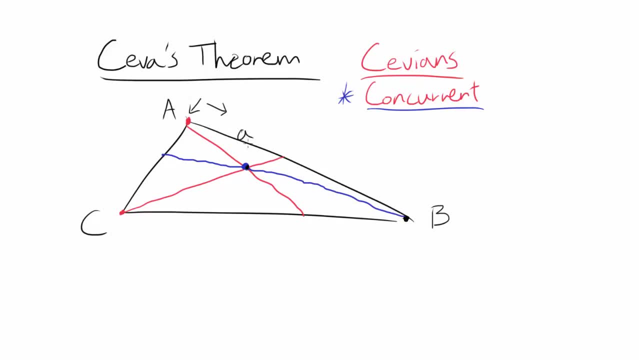 multiply. And you're going to start with: let's label some of it. Let's call this A, Let's call this B, Let's call this C, D, E and so on. And you're going to start with: let's label some of it. 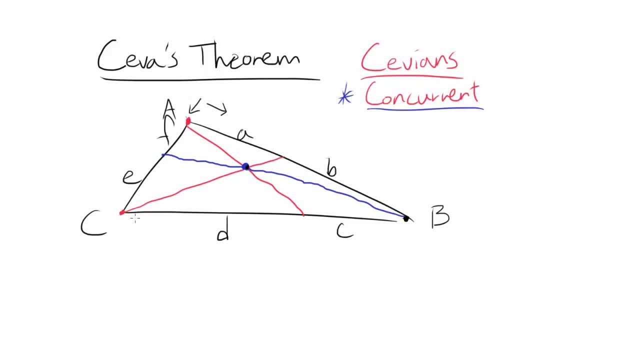 is C, D, E, F. So we have divided the triangle into six segments and what you're going to do? you're going to divide A by B and you're going to divide C by D. You're going to divide E by F. 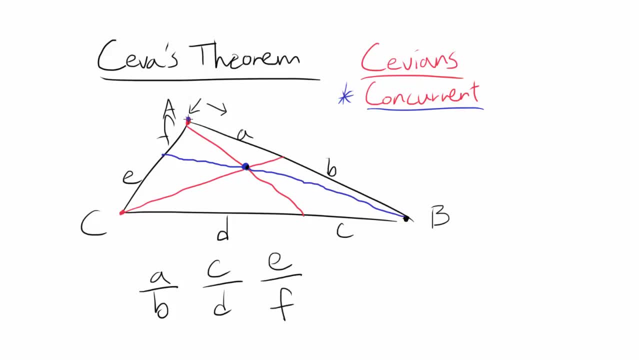 and maybe you're seeing. what we're doing is simple. You're starting at one vertex. You're just going around dividing the subsequent terms: A divided by B, C divided by D, E divided by F. That's all we're doing, and at the end you're going to multiply all of them together. 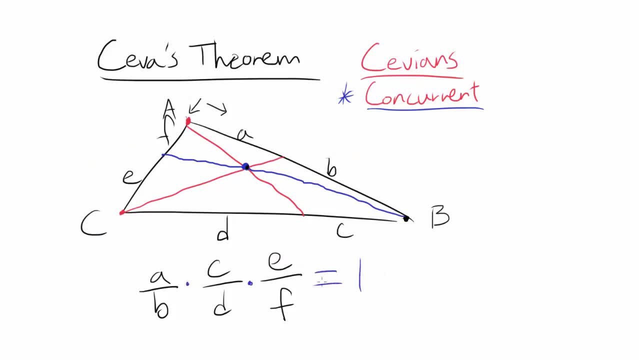 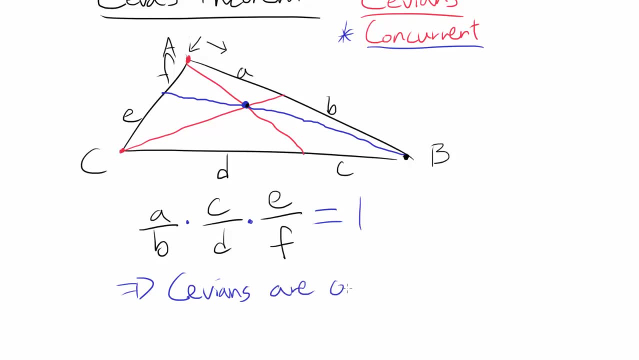 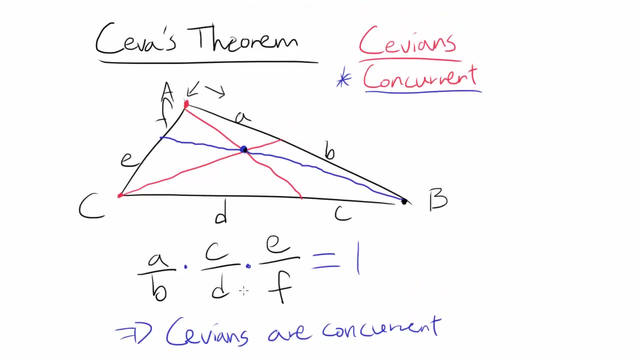 So you're going to multiply all of them together and if this thing comes up to be one, if this thing comes out to be one, then you know Cvn's are concurrent, Cvn's are concurrent, Concurrent, And the opposite. the converse is true as well, If Cvn's are concurrent. 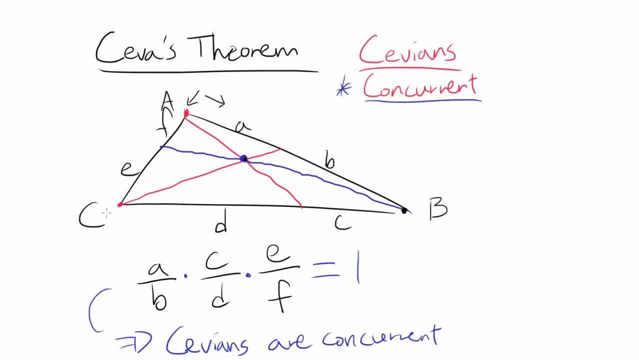 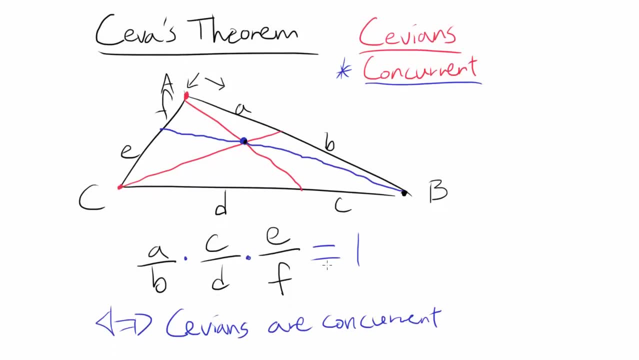 A over B, times C over D, times E over F is going to be one. So this thing works both ways. It's an if and only if theorem, Or necessary and sufficient condition. So Siva's theorem has immense applications as we are about.